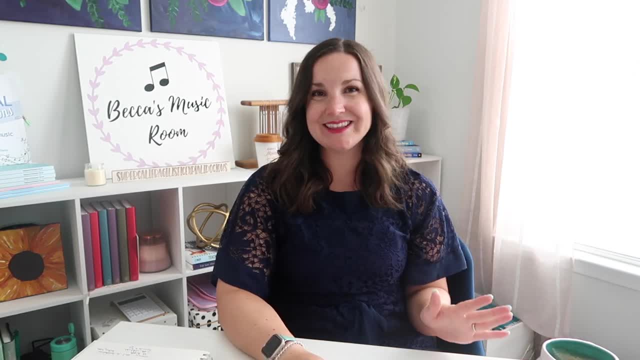 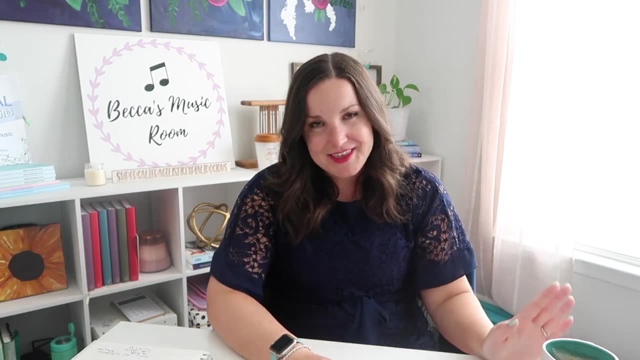 um, terrifying. but the good thing is the kids are forgiving. so I don't think any of them remember that, except for me, and it's so. after that I actually went and put some effort into it, into figuring out like, what am I actually supposed to do, what I'm actually supposed to say, and so 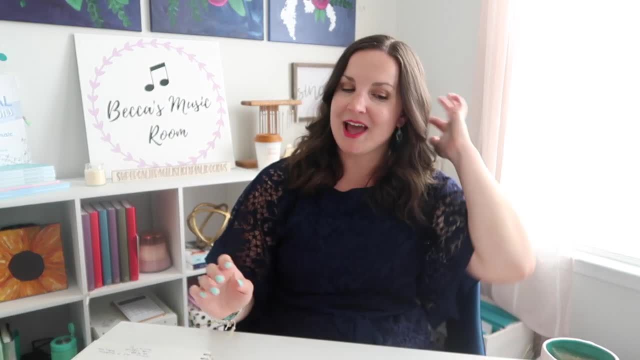 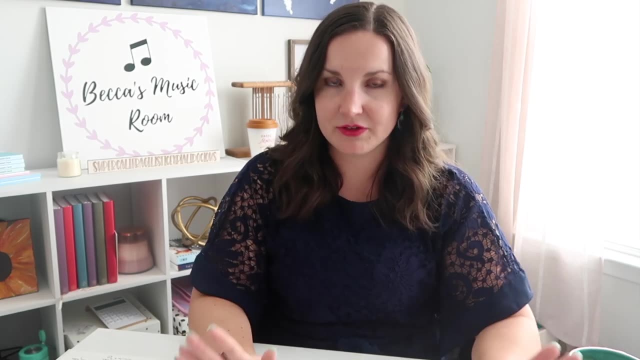 here is your answer to what you're actually supposed to do and what you're supposed to say. um, so we're gonna go through, step by step, how to teach rhythm. it's going to sound like a lot. don't freak out, because it's very like stepwise, so it'll be very simple. it's not necessarily easy. 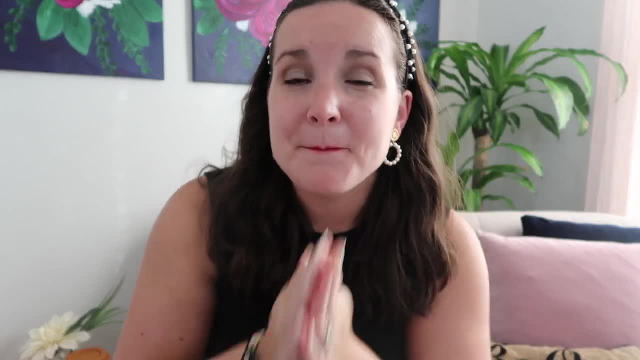 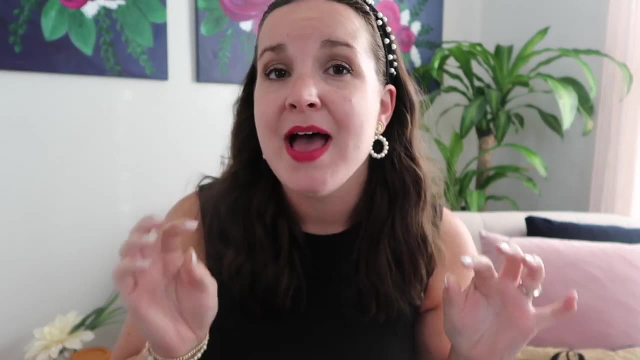 but it's very simple to figure out. sorry to interrupt your program, but I did want to let you know that I have a super special offer for my new elementary music teachers. if you are a new elementary music teacher, then you should click the link down below to get access to the free. 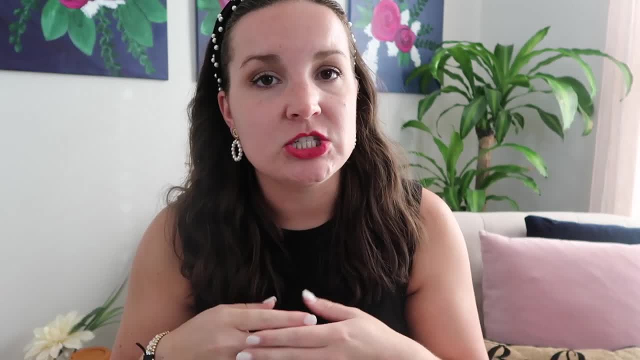 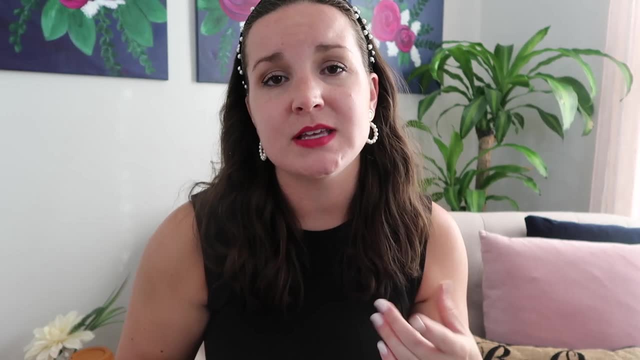 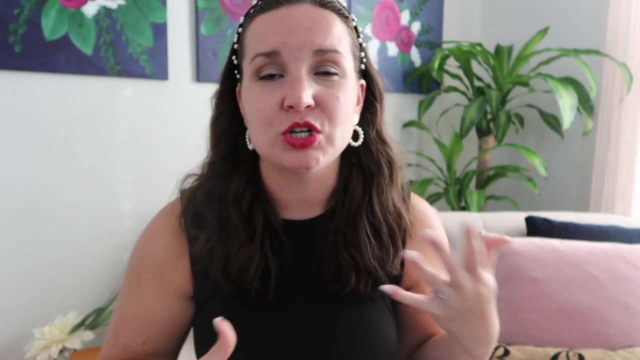 music teacher course. it's going to be seven days. each day you will get a video with the topic. it's short, the longest one, I think, is like 20 minutes and then a whole bunch of resources including blog posts, ideas, lesson plans, freebies, other videos to watch that are on similar topics. 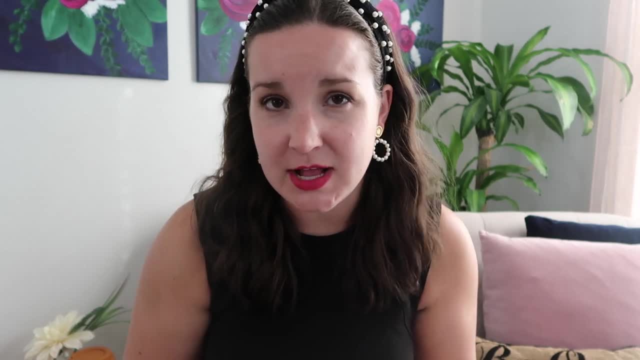 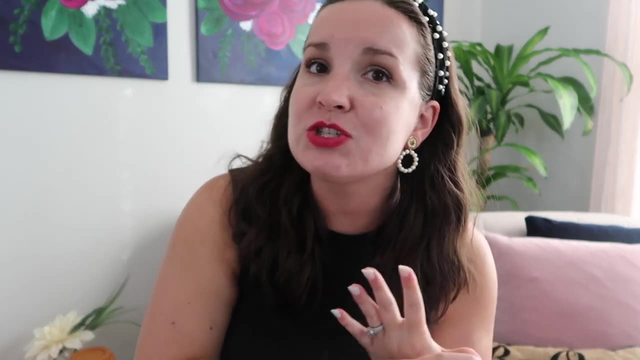 and things like that, so that you can really get a good grip on the basics of teaching elementary music. we're talking about what you should be teaching: how to create a scope and sequence, how to teach rhythm, how to teach melody, classroom management, how to structure your day and basically all the things that you should have learned in your 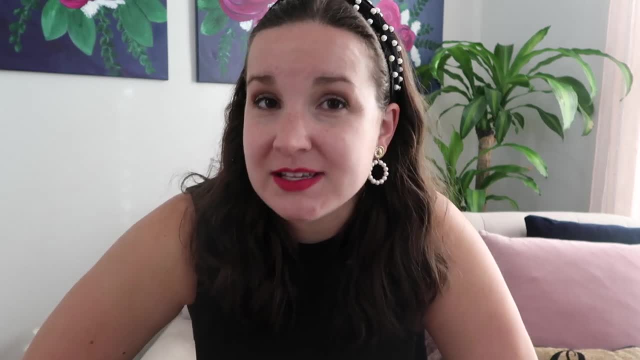 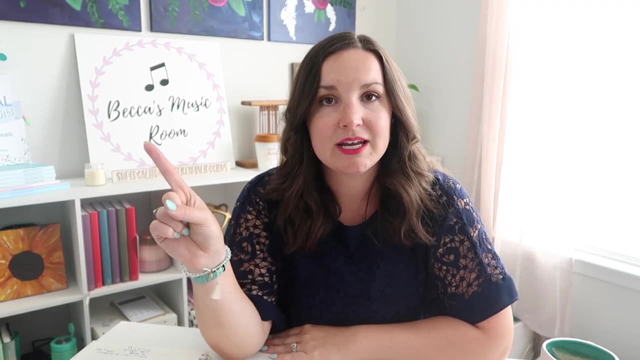 undergrad, but you probably didn't. so if that sounds interesting to you or helpful at all, you can click the link down below. it is completely free check it out. so step number one is steady beat. you need to start by making sure your kids know how to keep the steady beat in kindergarten. 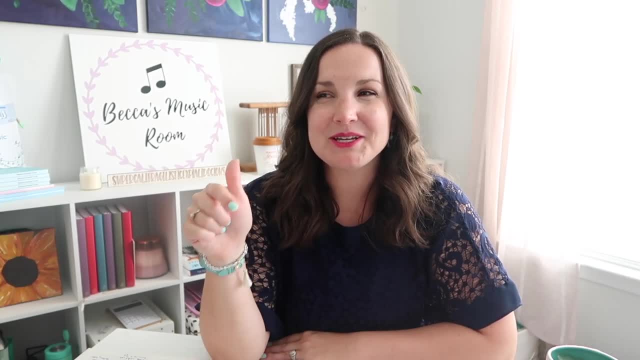 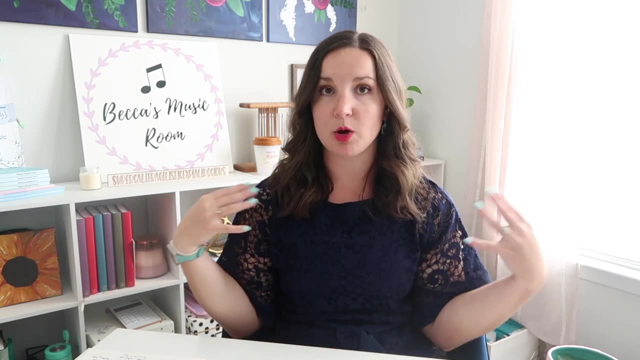 this is what you're going to spend like most of the year on um is there kindergarten at the first grade? you really want to get that steady beat practice. in order to do that. we're going to do it lots of different ways, so we're going to keep it on our bodies while we sing songs, while 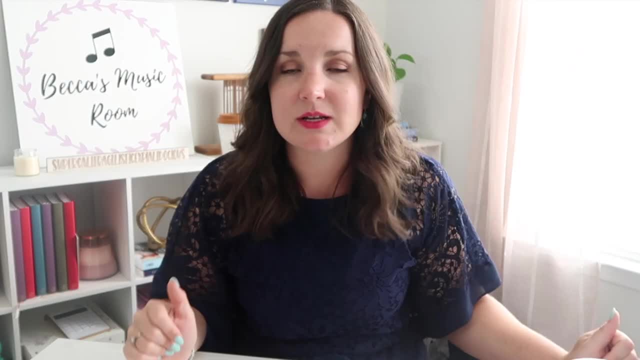 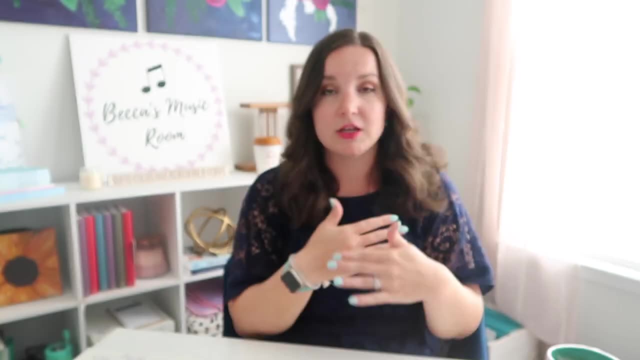 we listen to songs, we're going to keep the steady beat all over. one of the easiest way to do this is just stand in front of the kid and say: follow me. you know, and just keep going as you listen to a song or as you sing one of the songs that you're. 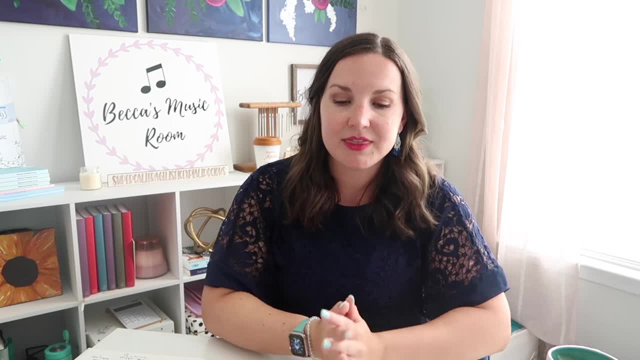 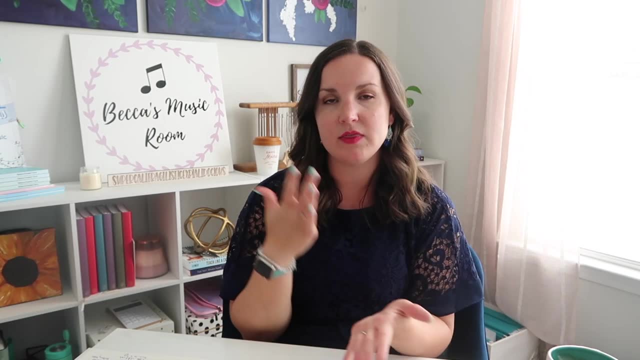 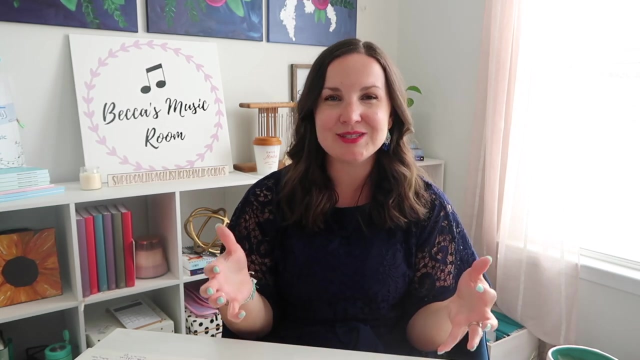 learning and keep that steady beat. um, along with that, another way that you can keep the steady beat, that's great, because the kids can hear whether they're on the beat or not. you always, i'm going to suggest, have a louder instrument up in the front, so like if they're all using hand drums. 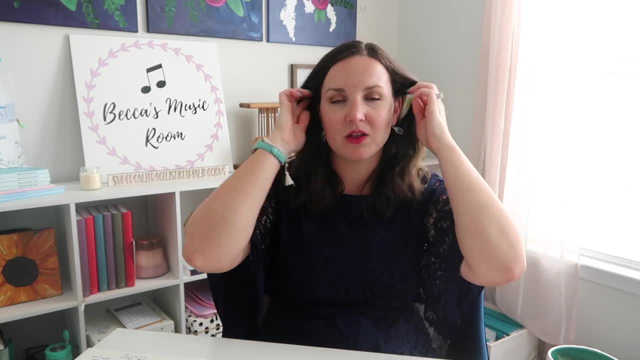 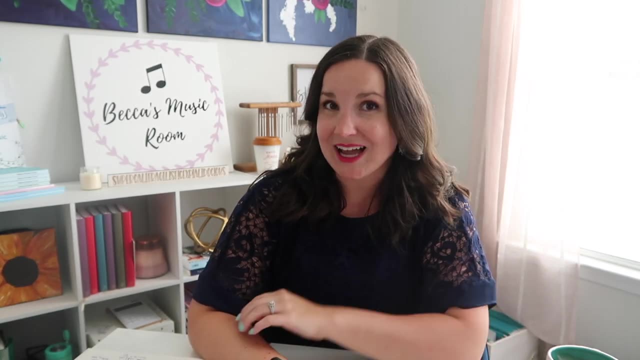 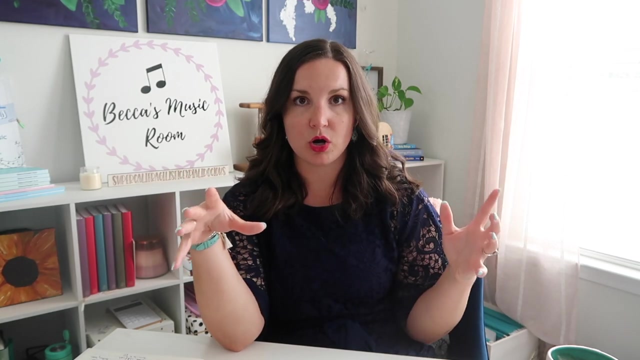 maybe you have your big djembe and you're playing the steady beat along with them a little bit louder so that they can hear it above all the rest of the noise. you can also do the steady beat by beat tracking, so that means that you have, like um, either cymbals or hearts on the floor or on the 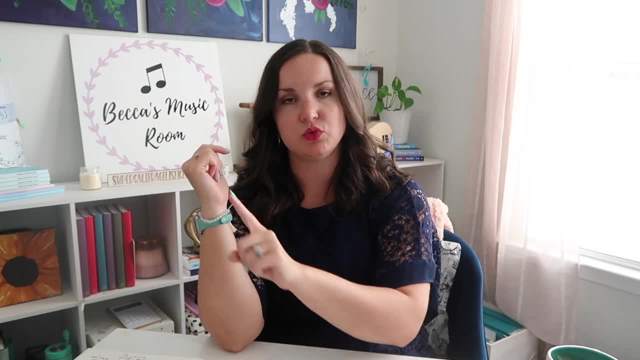 board that kids can actually play on the floor or on the board that kids can actually play on, the board that kids can actually play on the floor or on the board that kids can actually point, to point to as they're listening to the song. so this is- this is kind of actually the progression of how 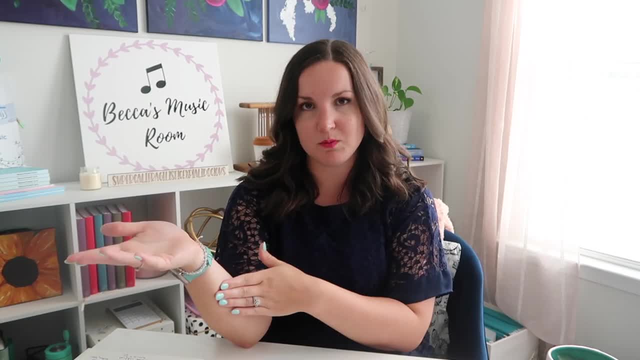 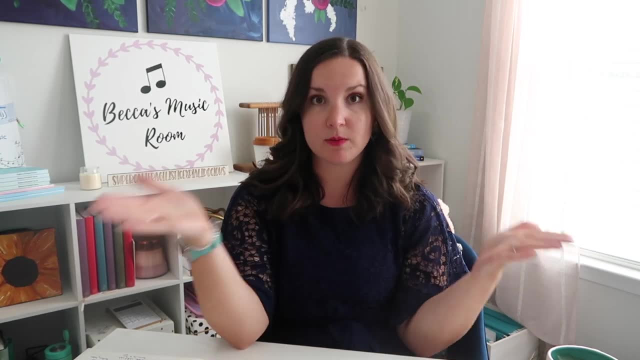 we would do. it is we would start with our bodies and then we would go to instruments and then we would beat tracks. so i would start by like pointing to them up on the board. sometimes that the kids can point to them on the board. i also have like heartbeat charts. actually i have 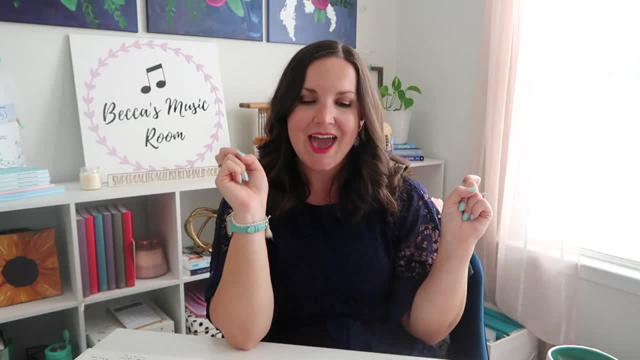 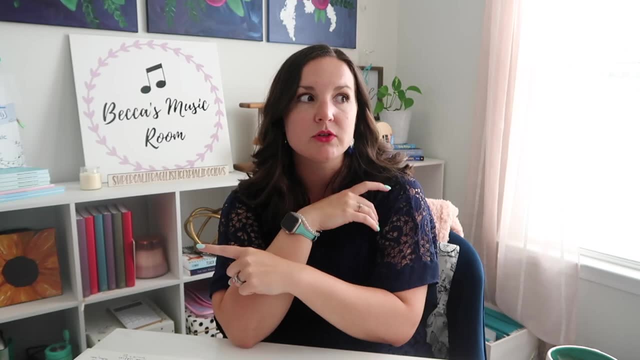 free heartbeat charts. oh, you click the link down below to get some free heartbeat charts, and so then you can, um, grab some heartbeat charts and have the kids you know point to the hearts. or if you want new symbols, so like if you're singing the song about elephants, you could do. 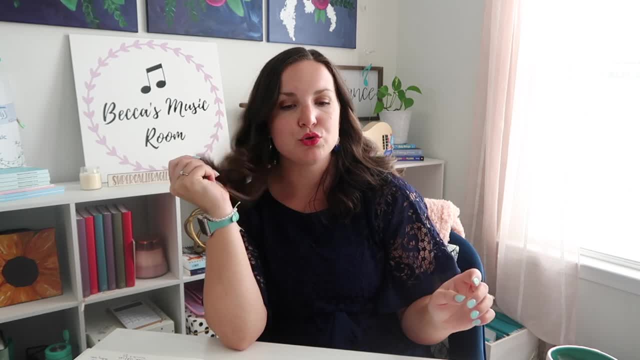 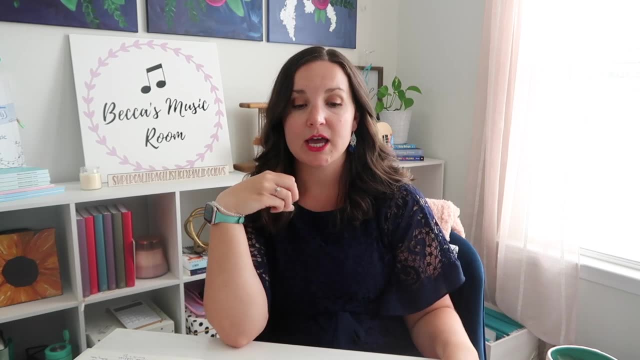 like little elephants. that's fine too, um, and then you can do some passing games, which is even more fun. so some of my favorite passing games are: bounce high, bounce low, akabaka and pass the shoe. so i will link those all down below so you can check those out. step number one is the study. 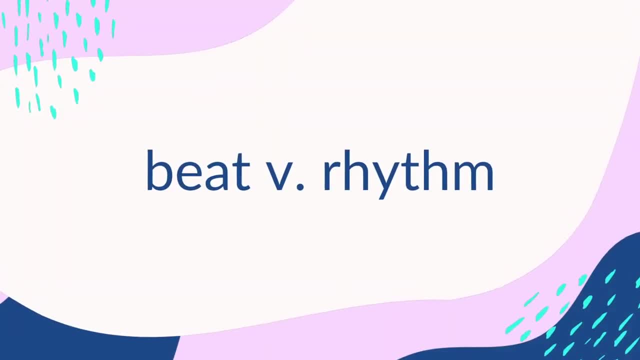 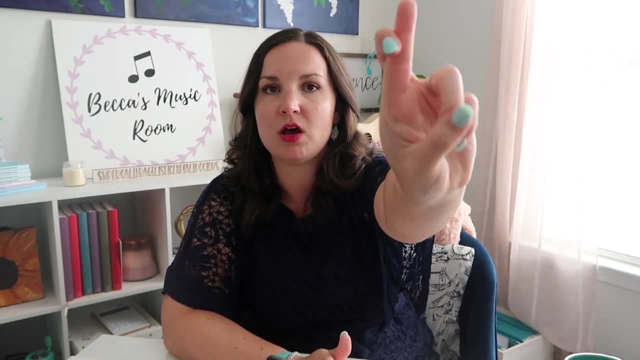 beat. step number two is beat versus rhythm. now i like to use the hand signs for like everything, and so we use b for b- this is a b in sign language- and r for rhythm. and my kiddos know that, like i mean, if i go to my fifth graders i'm like what's this mean? they'll be like: oh it's. 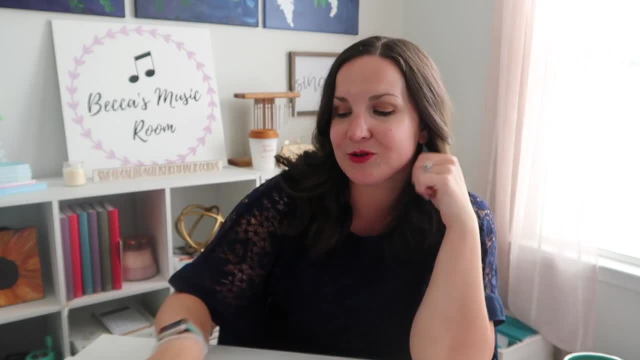 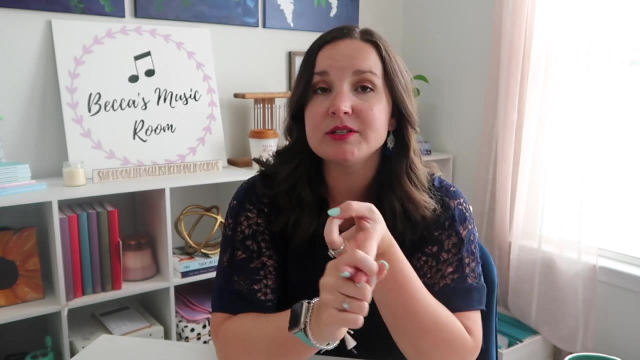 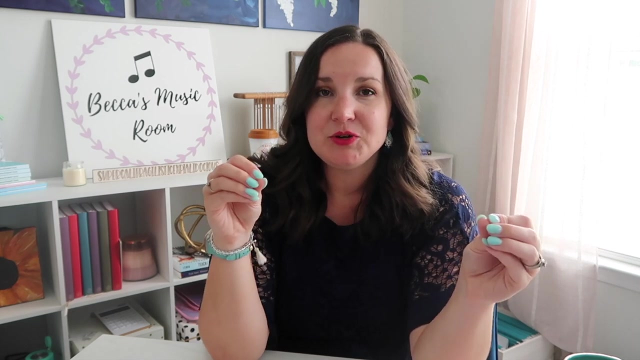 rhythm. yeah, you're right. so we talk about b versus rhythm a lot and specifically, we talk about how rhythm is the way the words go, it is the syllables, and rhythm is long and short notes. so those are like the three things we always say about rhythm. the first thing you want to do is compare it to. 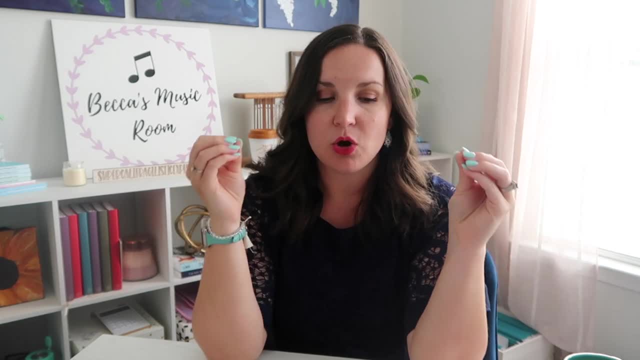 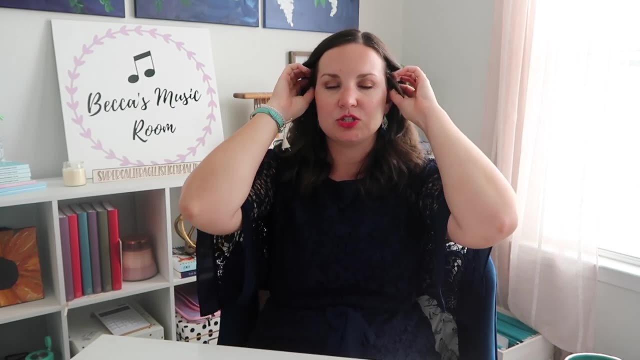 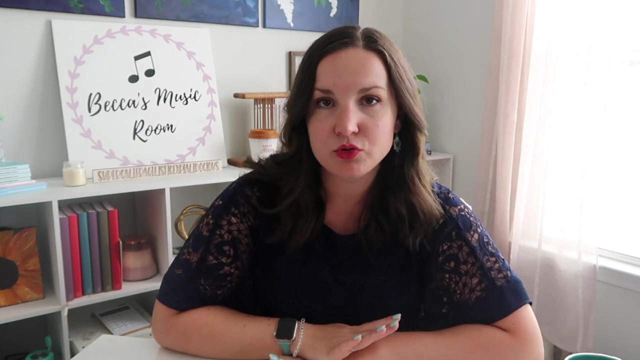 how the words go or the syllables. so i usually end up teaching this in october, which is great. there's this really fun k music k8 song called hey jack and it's super, super cute, and so with this song the chorus goes. so what we do for this one is we play the rhythm on the chorus and then 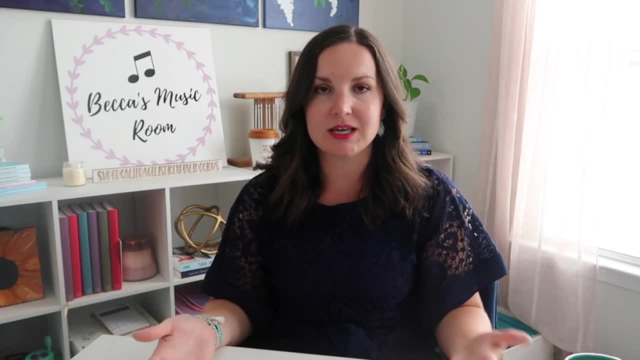 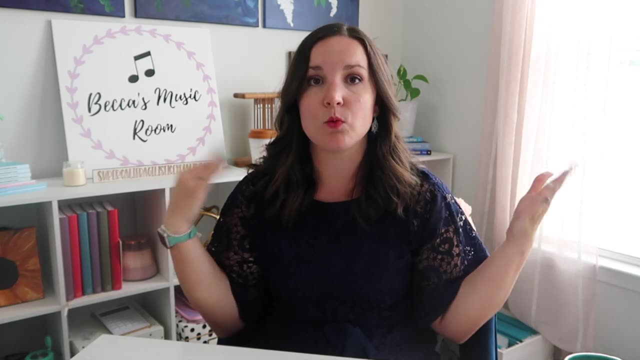 the rest of the time, we keep the steady beat around our bodies, and so it really gets that like beat versus rhythm thing going on. we also, just like when we're singing our songs, we'll play the steady beat and then we'll play the rhythm, and so we can feel the difference. we'll 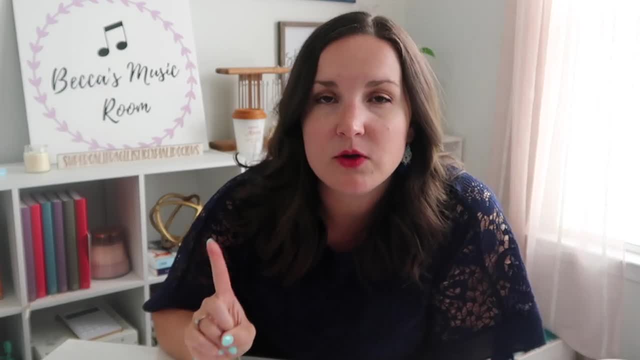 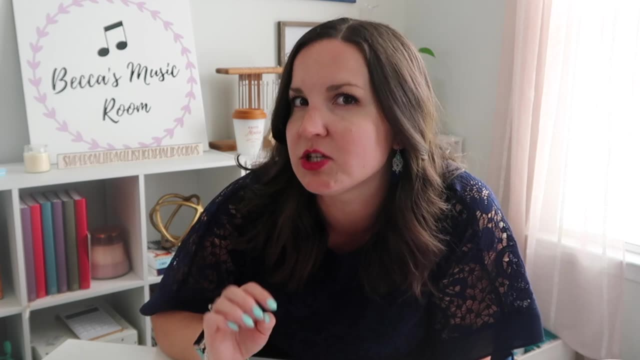 play them with instruments. there's also a go noodle video. if you haven't learned about go noodle yet, it's amazing. go noodle is um like fun brain breaks for your kids, but there's lots of like songs and dances and so there's one of the go noodle videos that's about syllables. it's called. 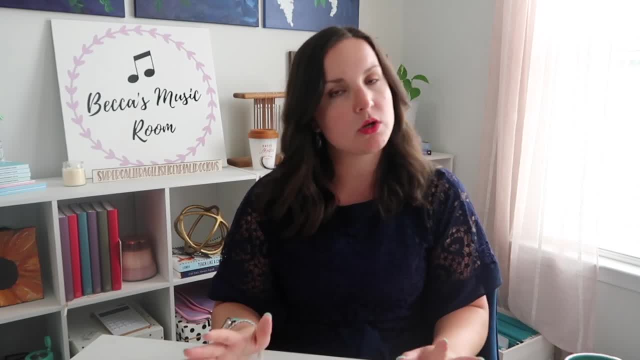 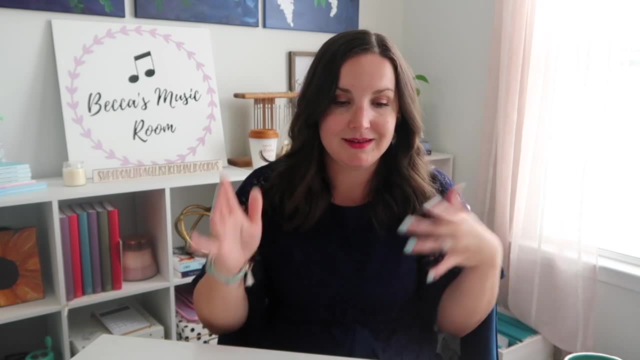 clap it out and so they're clapping syllables. so i love to do that one when we're learning about rhythm, so that we can clap out the rhythm and we'll talk about how the rhythm is clapping of syllables and all that stuff. and yes, first graders know what the word syllables means. 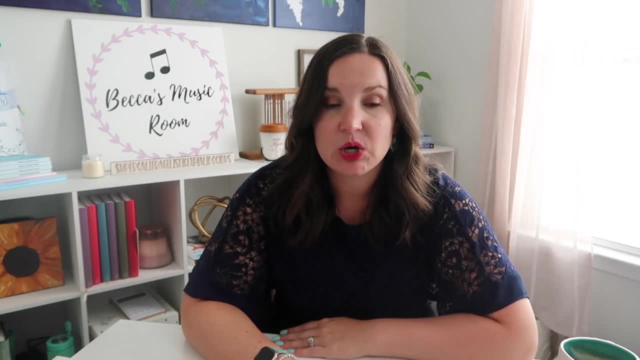 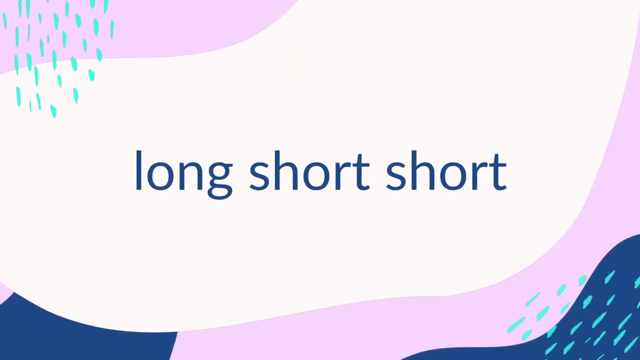 and then they'll say: that's great. now, this is all before they have ever even seen a quarter or an eighth note. by the way, instead of quarter and eighth note, we're gonna start by calling them long and short, short, or you can just go straight to ta and titi or tah and tatty, however you want. 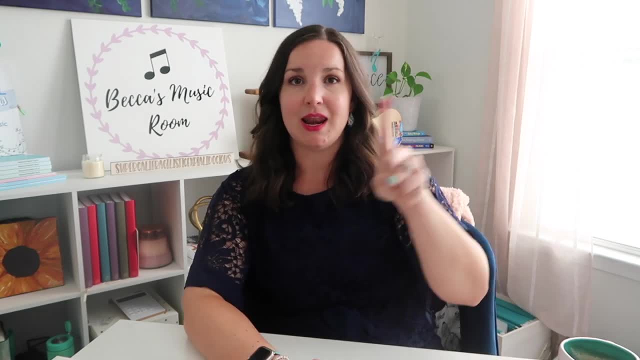 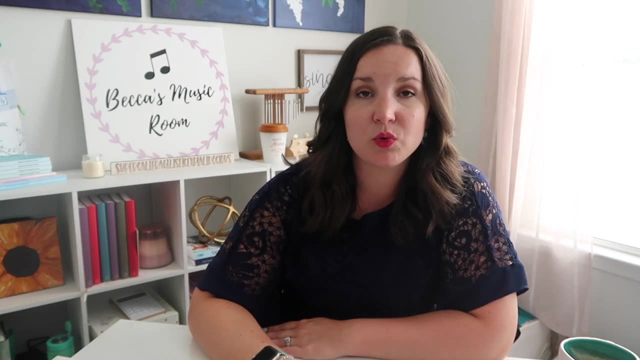 to do that. but long and short short is really helpful because you can do like line and then like dot dot for short, short, so you can get the kids writing and reading before they ever actually look at a quarter note. you can also have them echo things so like when we learn a new song, i'll you. 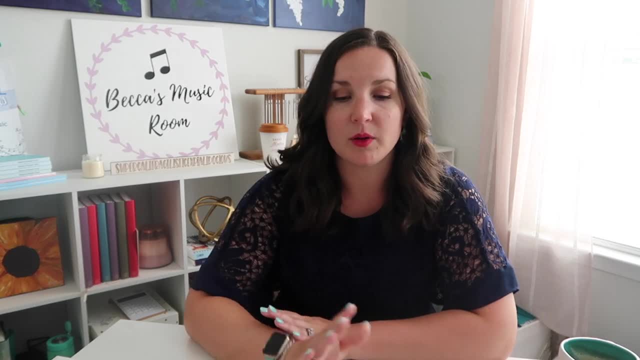 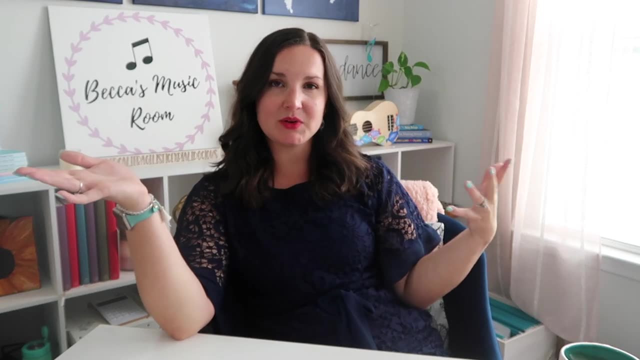 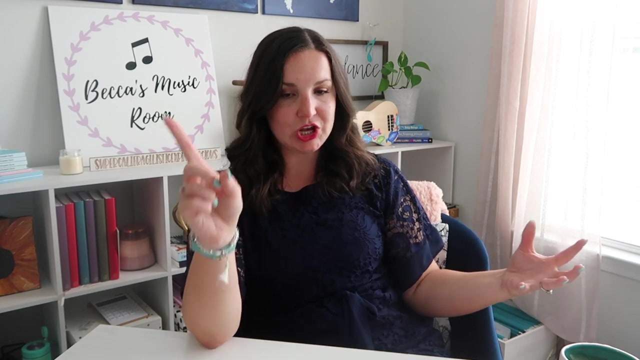 go the rhythm, so we'll be like ta, ta, ta, ta, or play the rhythm, or you know long, long, short, short, long or whatever. we're gonna do all right, now that we actually know, you know, the difference between beat and rhythm, we're gonna put sounds onto the beats, okay. so what i mean by that is: 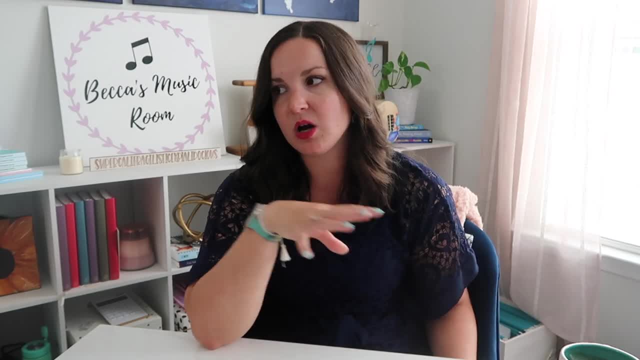 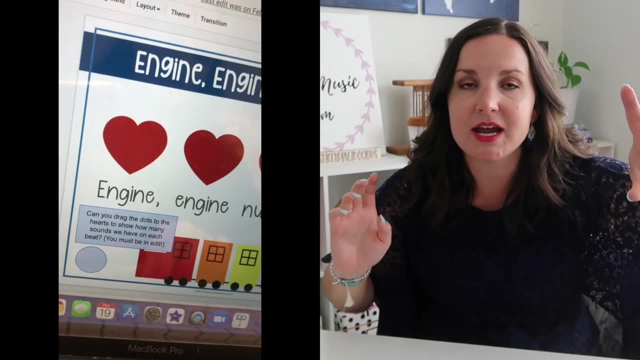 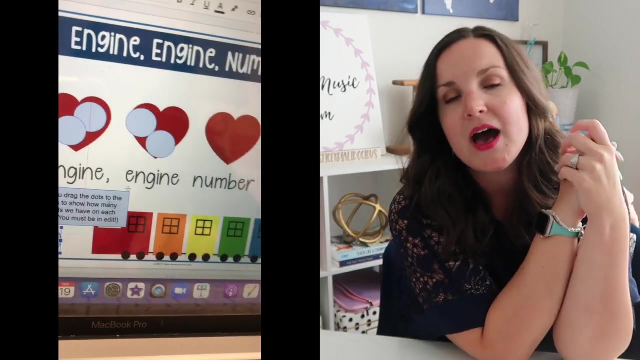 that you're going to want to have some sort of like heartbeat chart. we always do this together first, so i'll put hearts up on the screen and we'll figure out that if i put one dot, it's gonna be, you know, ta or long. if i put two dots on the same heart, it's gonna be tz or short, short. i did. 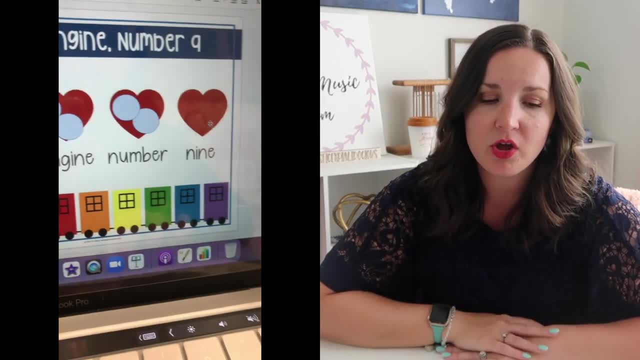 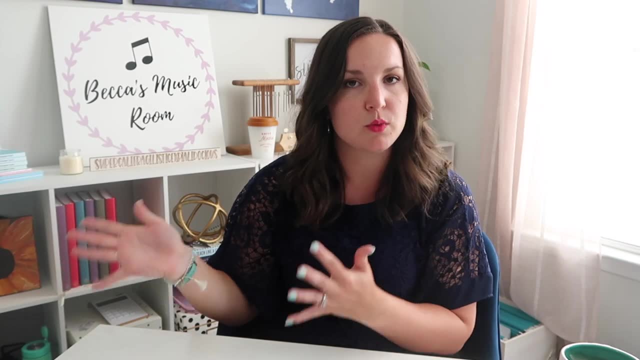 this this year with engine engine number nine and it was super helpful. i will leave a link to the youtube video to engine engine number nine and like how i did that and taught rhythm like the whole way through with that one um. it's a really easy chance. so definitely check that out, but it 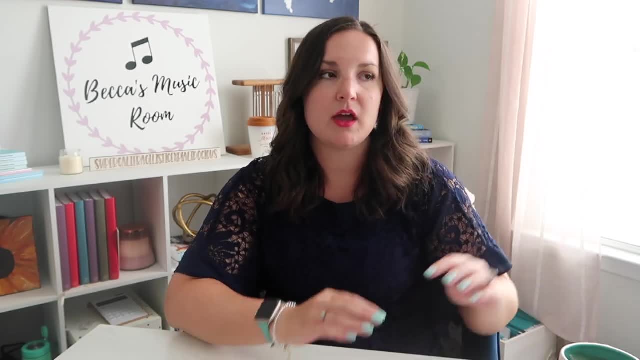 really helped me to be able to show them how to play the rhythm and how to play the rhythm, and how to play the rhythm and how to play. so we could figure out like, okay, and gin is under the first part, so that's two sounds, that's two. 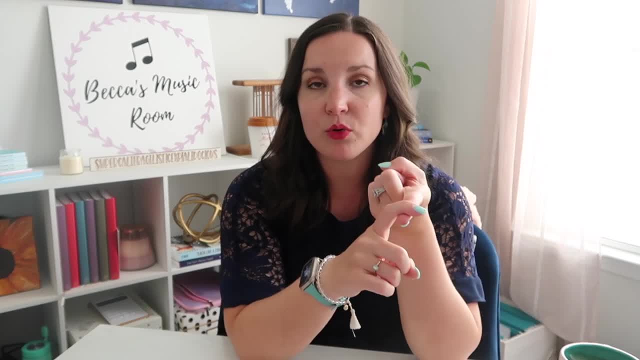 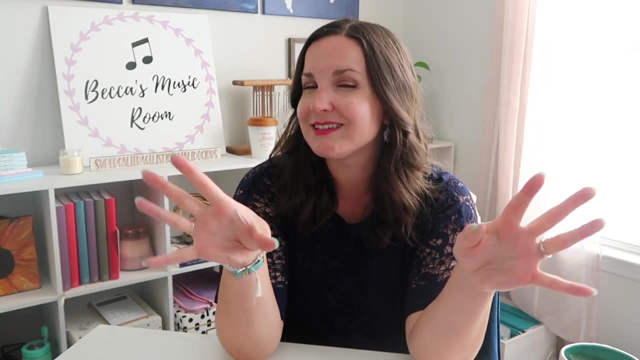 syllables. so we're gonna put two dots on there so you can do that up on the board, you can have, you can do it on the board. after you do it on the board, you could have the kids do it themselves. and one of my favorite things is to do chair rhythms. so we'll put four chairs front and we'll 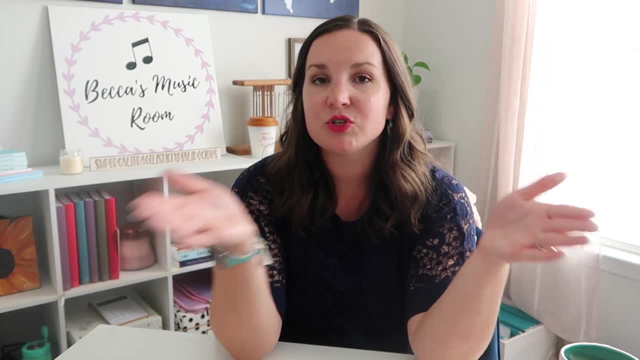 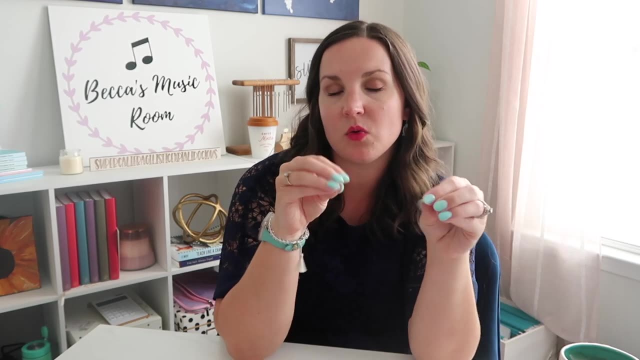 have a kid sit in each one, and then i'll have two kids in some of them. so if there's one kid, then it's a top or a long, and if there's two kids then it's tt or short, short. so you'll have and it's a. 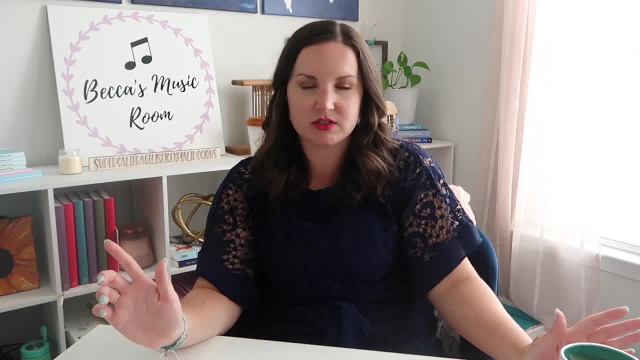 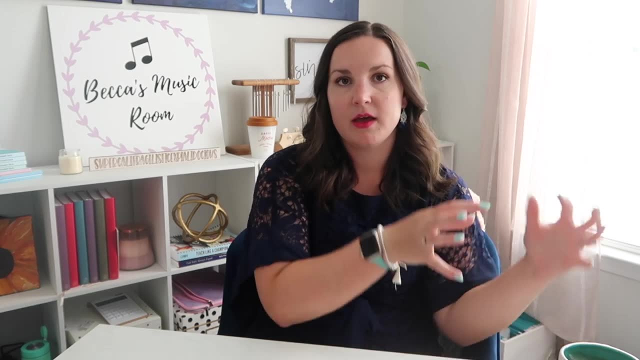 really like physical way for the kids to see it and also it's like silly, so they just love it and it's great, um, and it's a lot of fun, and they can see, like, okay, the chair is the beat, how many kids are on there. you can also do this, by the way, with stuffed animals. that's a lot of fun too, and i'll 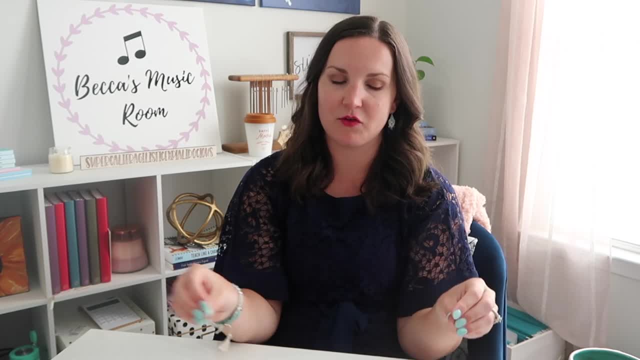 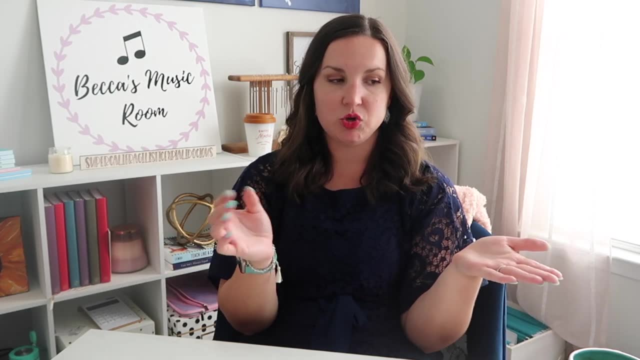 have the kids come and like arrange the stuffed animals, so there's like one or two or however many. so much fun and they love it. and then you can also do: you take those same printables that i already linked and you can have them put um manipulatives on there. so you can get mini erasers or bingo chips and have them put. you know two. 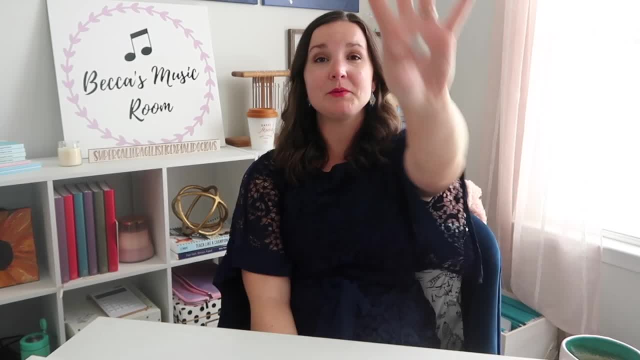 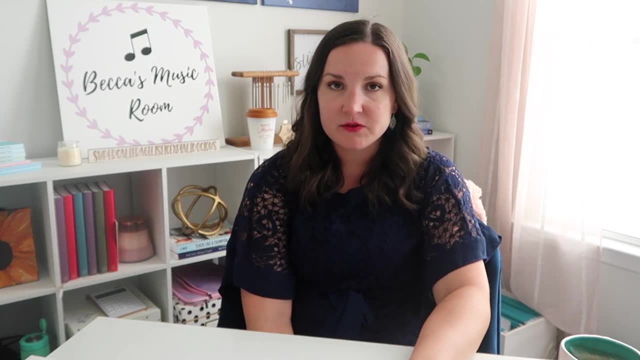 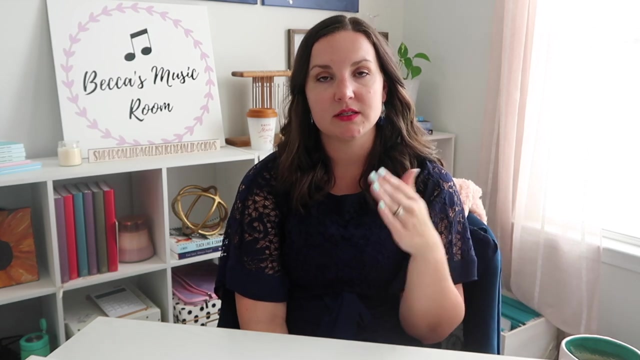 bingo chips on a heart if it's td and one if it's top step. number four is gonna be introducing the rhythm. yep, three steps to get to. so i use taught and tt for ours. um, you can use whatever rhythm syllables you prefer, but that's just what i use um. so taught is a quarter note and then tt is. 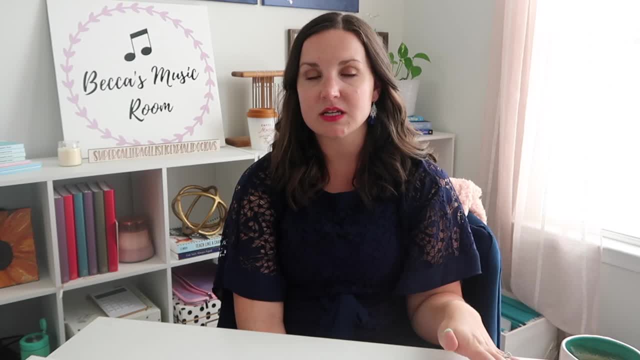 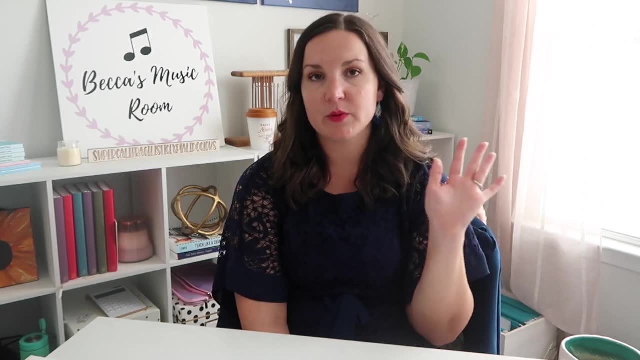 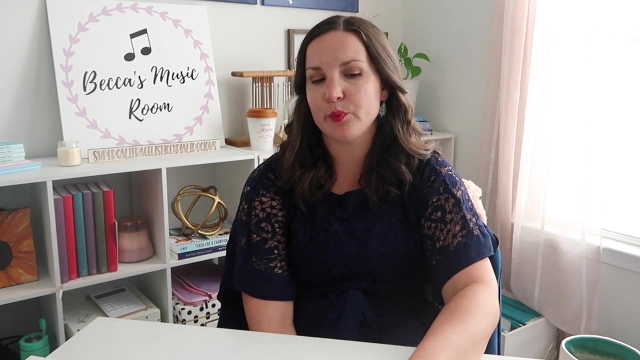 eighth notes. i do not teach them the names until they get to about third grade, so the little kids just call them taught and tt and that's it, um, and we'll put them up on the board. you can also use stick notation if you prefer stick notation. i don't bother with stick notation because i don't think. 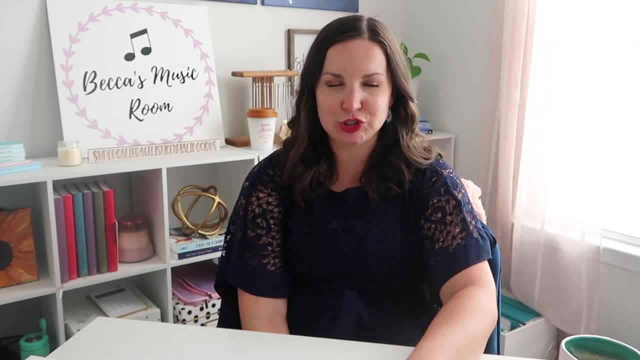 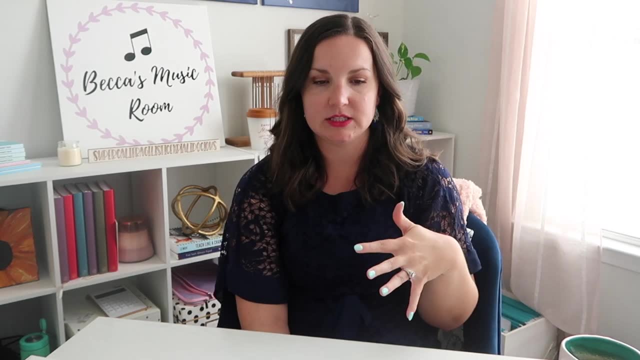 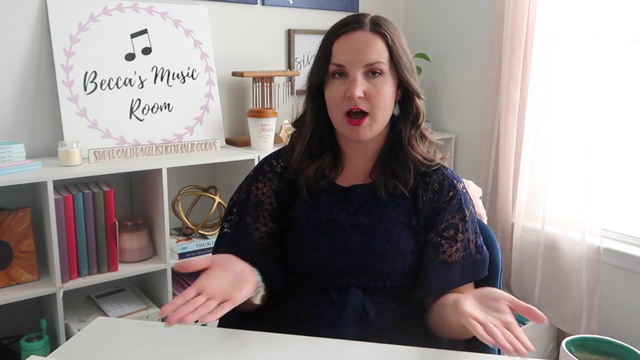 it's any easier than regular notation, so we just do regular notation after we have learned what the rhythm is. then we're going to start with reading and pointing. so now we're going to put you know rhythms up on the screen and we're going to point to them and we're going to read them and we're going to have flash cards and 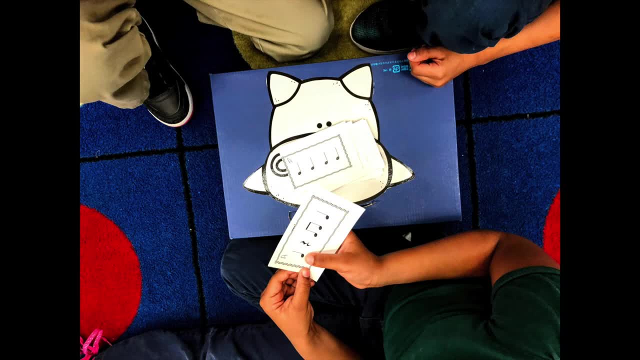 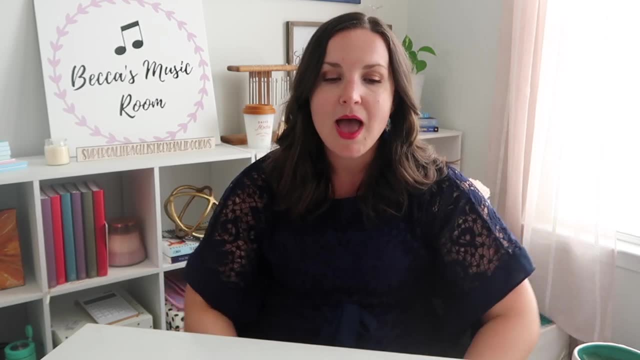 we're going to, you know, read them with our friends, and we're going to point to our own rhythms on our floor and all that kind of stuff. and, by the way, i have a free set of rhythm flash cards that i will also link down below, and so we're just going to start with like reading and 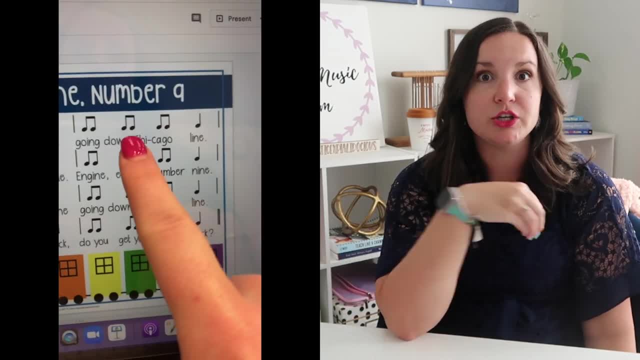 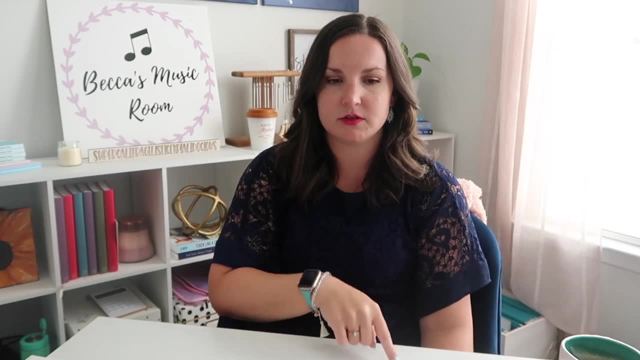 pointing. you can do um play along. videos on youtube are great for this, but just the idea being like we're putting them on the board and then we're going to start with reading and pointing and we're figuring it out and we're, you know, having that ta, ta, ti, ti, ta. different things like 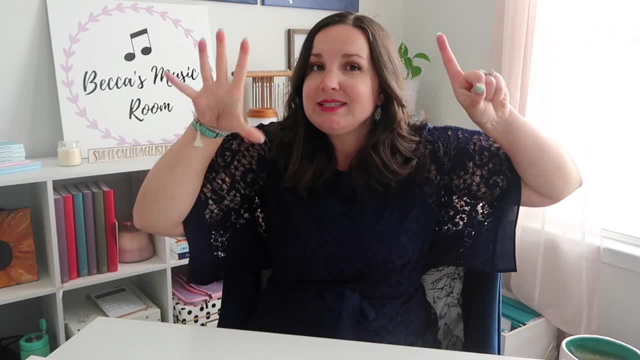 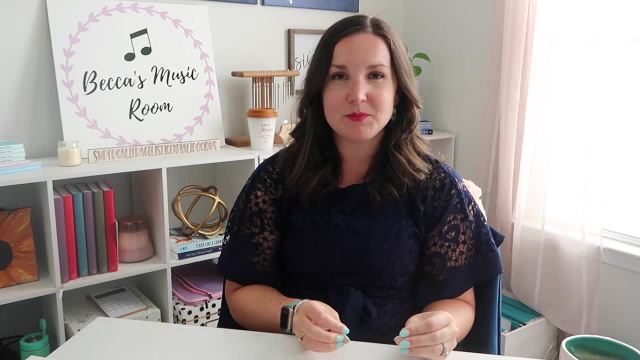 that that we're really starting to like understand. then step number six is we're going to start making rhythms. so whatever you're making is like actually making. so you want to use your manipulatives in order to do this. so a couple ways you can do that: um, you can get manipulatives. so 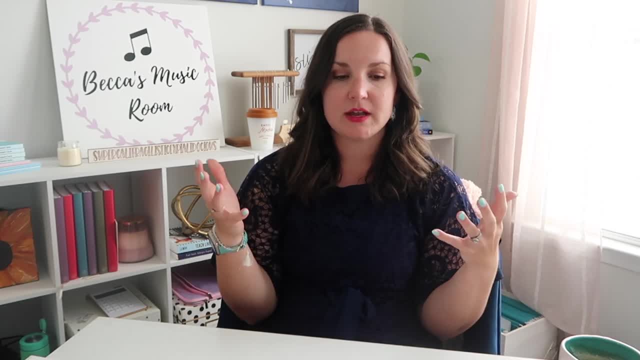 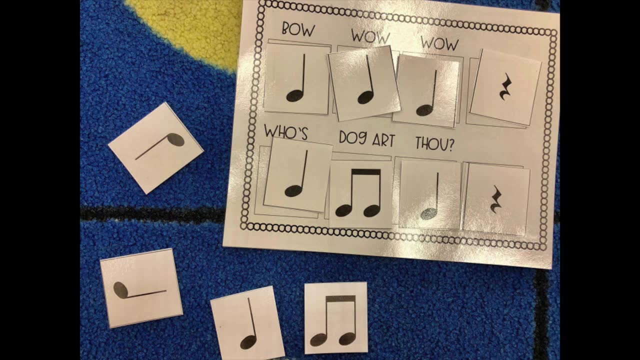 manipulatives are anything kids manipulate. um, you can do some like quarter and eighth notes on you bunch of them- and then print it out and have them use those in order to create different rhythms. i love doing this with the song bow, wow, wow. so i will link that down below so you can check that. 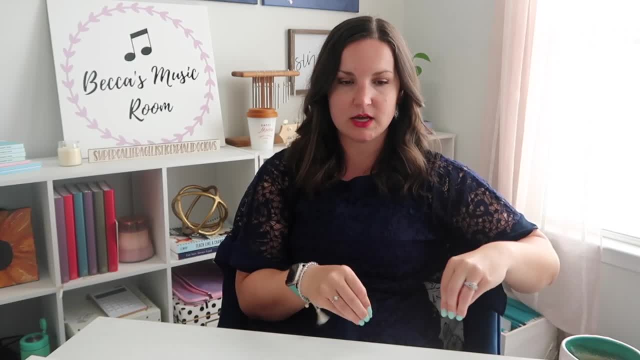 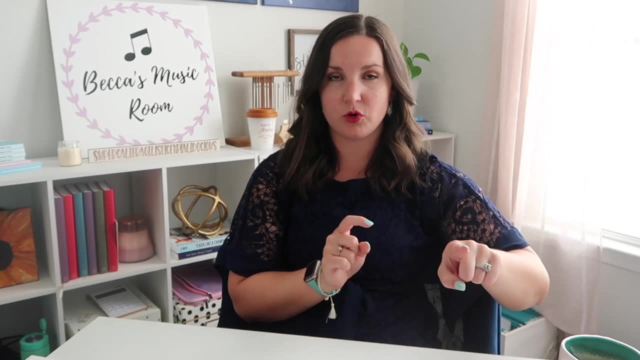 one out. it has printable manipulatives in addition to the everything else. popsicle sticks are a lot of fun. we use popsicle sticks in order to create rhythms, so we use one for quarter notes and then three for eighth notes. so it's like up and then one this way and then one this way. 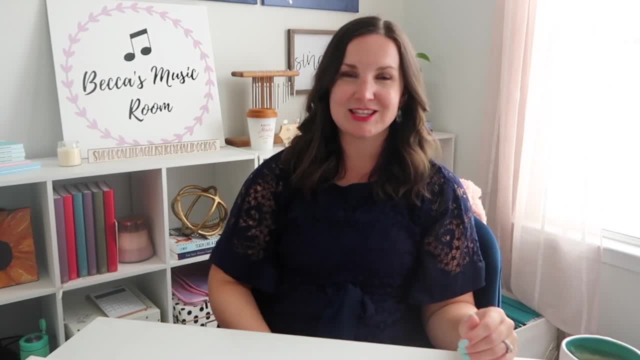 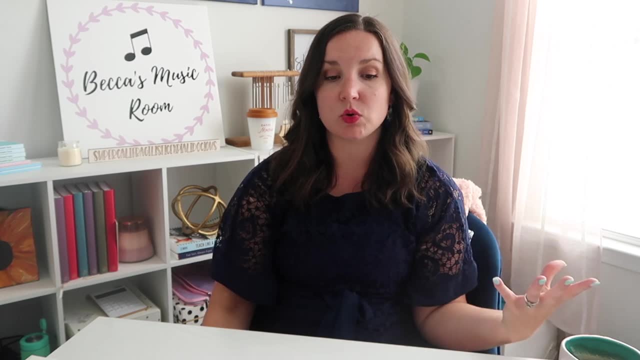 to make- and we call it like a house, um, to make the house for the eighth notes. so you can do them that way, you can do dictation with them. so have them figure them out. you can have them write on boards or have them write on paper or any that kind of stuff. 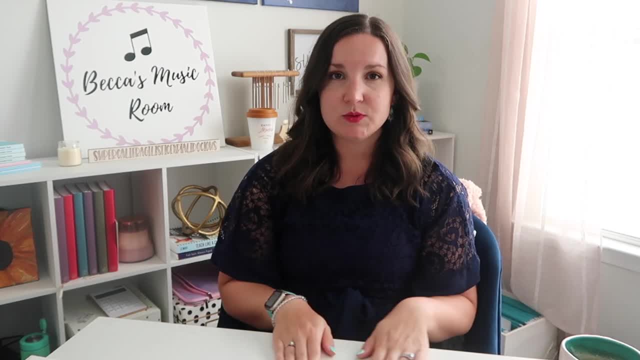 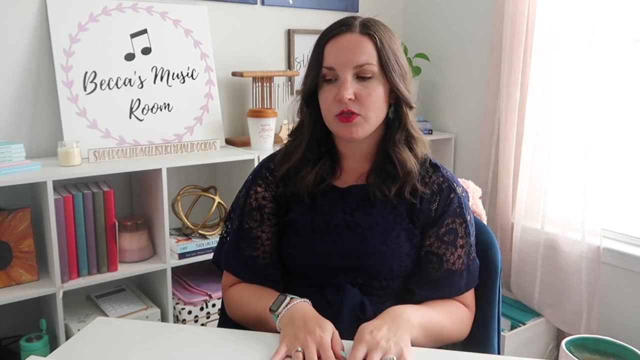 those are all different ways you can create rhythms. so what i like to do with these is the first time i'll give them, whatever we're doing- manipulatives, popsicle sticks, boards, whatever- and the first time i'll like tell them there then. so if we're doing ta, ta, ti, ti, ta, i'll. 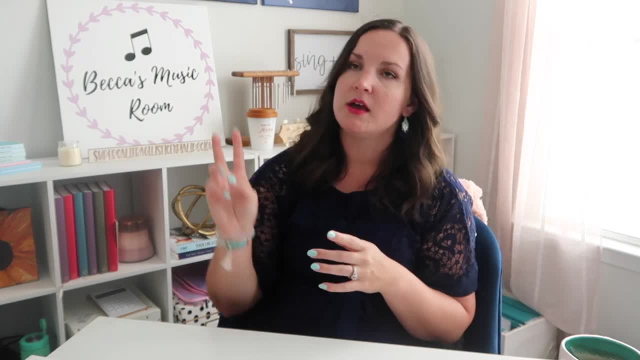 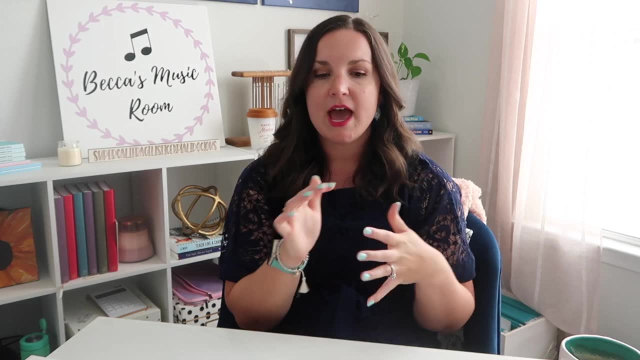 be like: okay, let's see if we can make ta, ta, ti, ti, ta, and i'll help them with that. and then i'll help them with the first one and write it out or put the manipulatives up on the board or whatever. and then the second time i kind of give them like a head start, and then the third time i'll give. 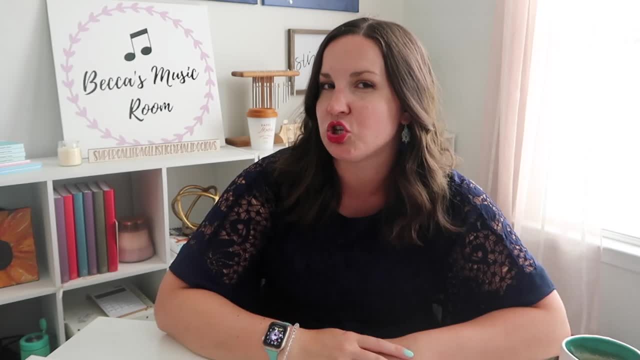 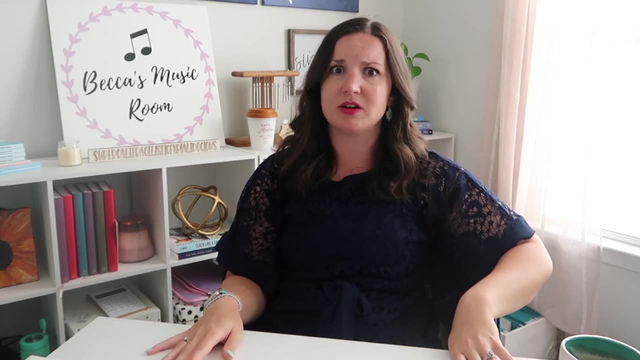 them even longer of a head start. so when you try it first and then i'll show you what the answer is, and then by the end of usually the first day, they can figure it all out on themselves. like the kids are smart, they'll get it. if you really prepared them for it, they will get it really. 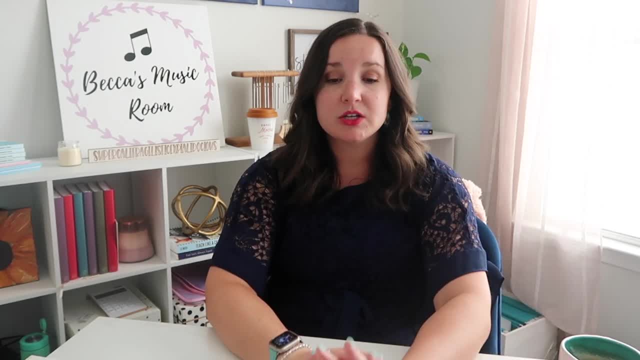 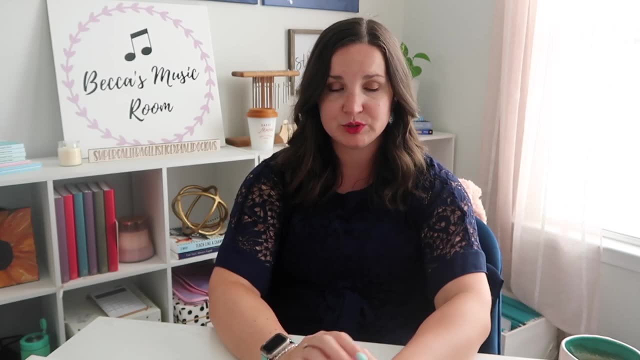 quickly, um, so that's really easy. you can also do this online with google slides, um, and, or on it near pod, and i will link both those options down below for you too. after we've done a couple of practices, then we'll start notating our song, so we might take that engine, engine number nine, and we'll 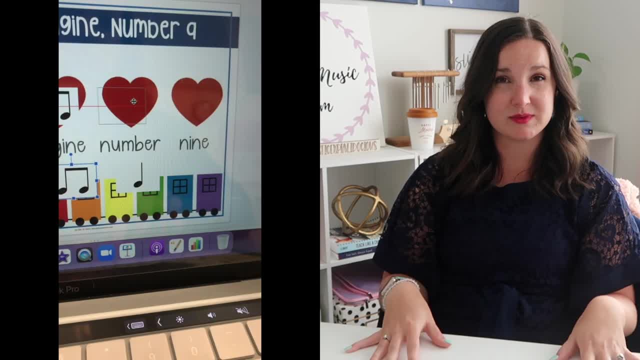 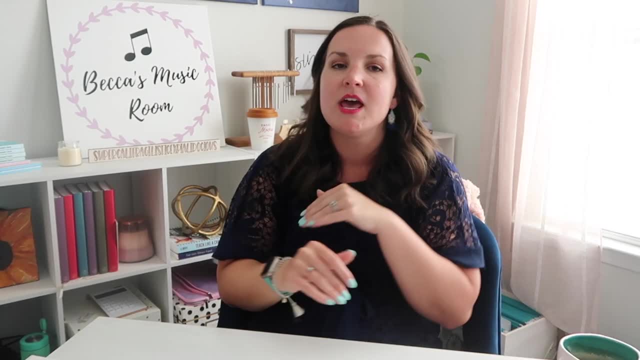 figure it out as a class and then i'll even have the kids figuring it out for themselves. so i always like to start with the class. so we'll put it up on the board and we'll you know like engine it's, like, which one does it match? and they'll you know kind of help me, and then maybe like the second or the 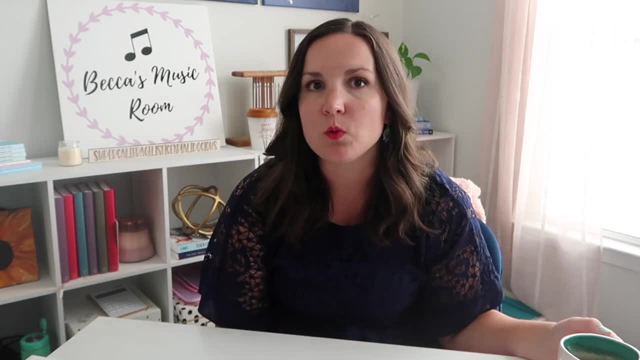 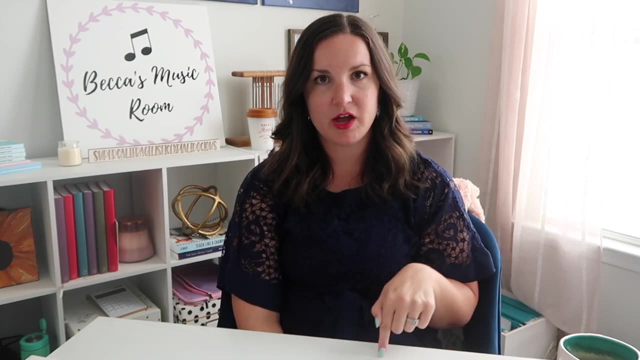 third line: they can do on their own, or they can, you know, fill in one of the missing ones, and i love to do, um, give them a song with rhythm on it and have like a couple of the rhythms missing. that's a great way to do assessment. just have a couple of them missing. they just have to fill in the empty ones. 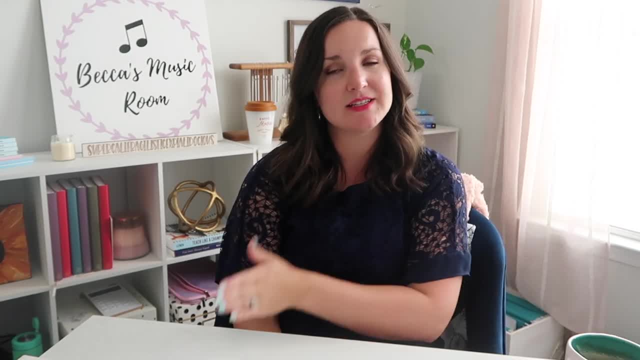 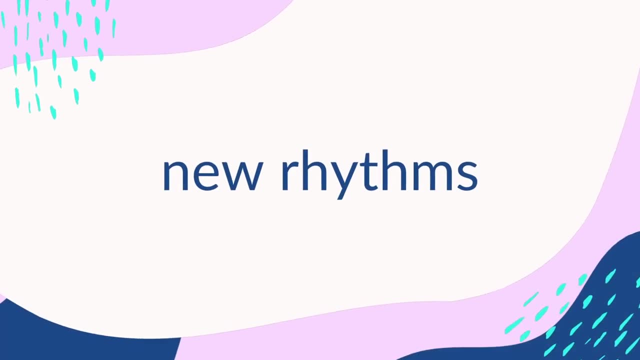 it's great. so, along with writing your rhythms, you're going to want to eventually have an assessment to make sure that they understand the rhythms. um, and then step number seven is going to be to add new rhythms. so the good thing is, you don't have to do quite as much work when you get. 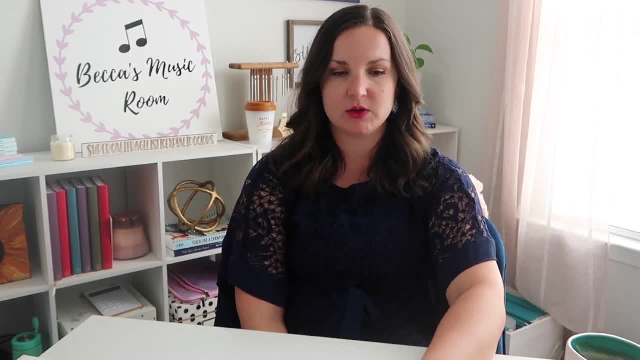 to the next rhythm. but you do still want to have some of the same steps. so i would still do with all of them, uh, figuring out how to do them. and then i would still do with all of them, uh, figuring out the sounds. how many sounds are on a beat, you know? so, like 16th, notes are talky. 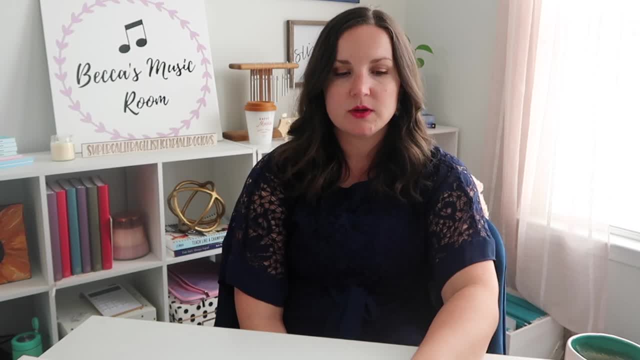 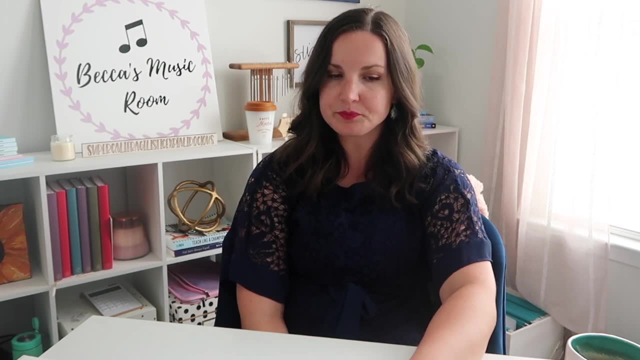 cheeky, that's four sounds on one beat. um, introduce the rhythm. you're still going to do pointing and reading and you're still going to want to make the rhythms and play them on instruments also all throughout. but you don't have to do quite as much work because they now at least understand. 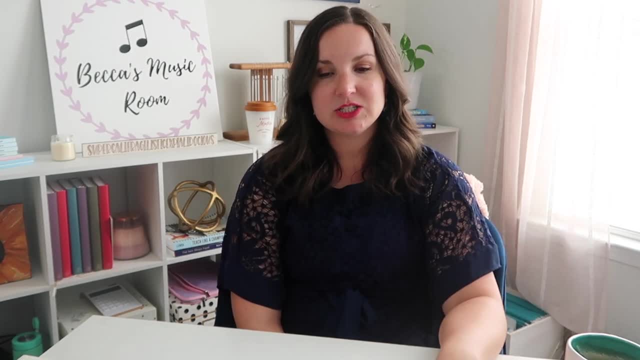 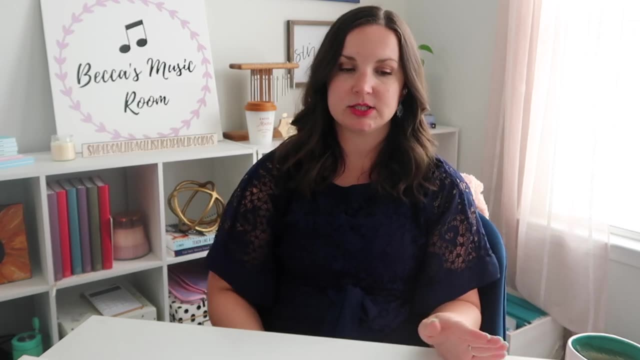 what rhythms are. so i usually do the order of. so if you're like, okay, what rhythms do i do? um, you can do them however you want, whatever your state standards say, but my order is always quarter and barred. eighth notes first, and i do that in first grade, then we do quarter rest also. 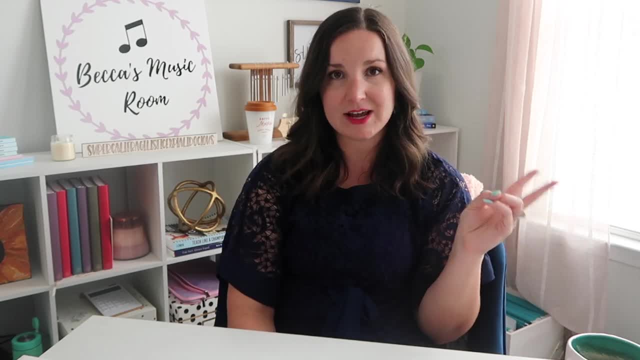 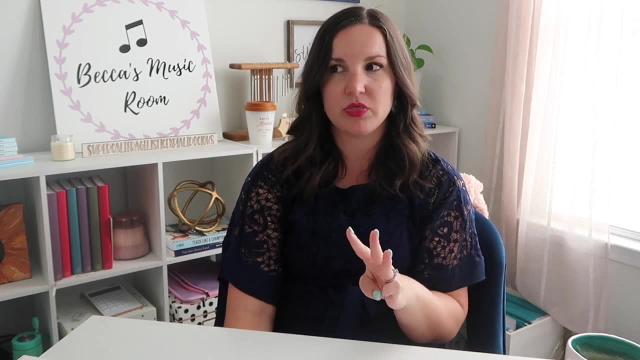 in first grade, um. in second grade we do half note and half rest. in third grade we do barred 16th notes and dotted half notes, and also in third grade i teach them the real names for everything so that they actually know what they are. and we talk a lot about like beats per measure. 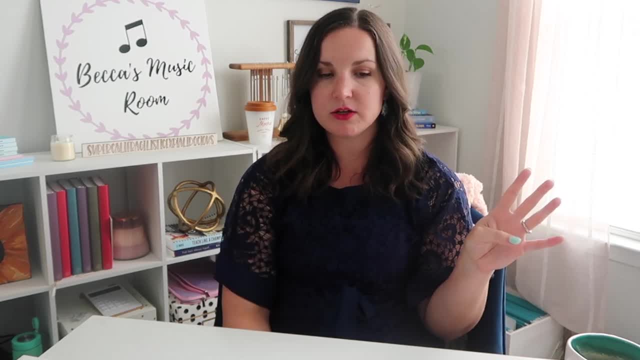 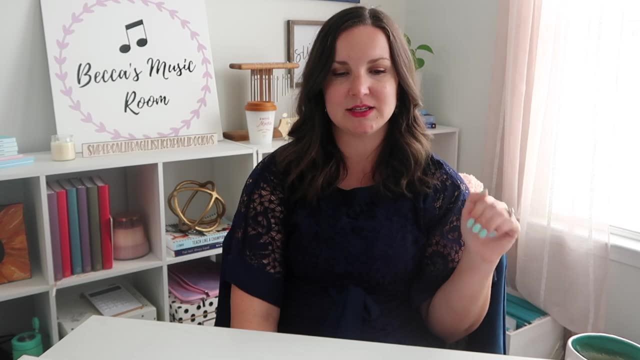 in fourth grade, um, we usually do a dotted quarter note and single eighth notes and whole notes, whole rests, and then in fifth grade, if we get to it, hopefully, we get to do triplet and cinco pop, which is eighth, quarter, eighth, and that's usually as far as 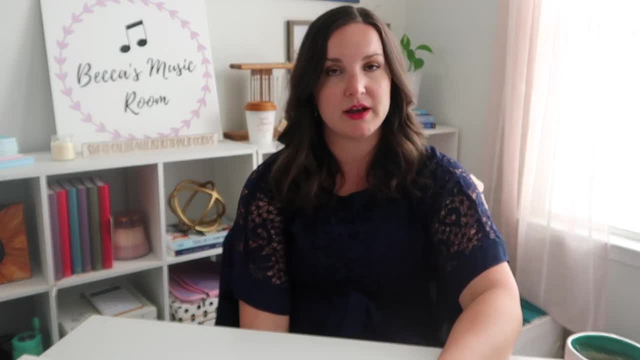 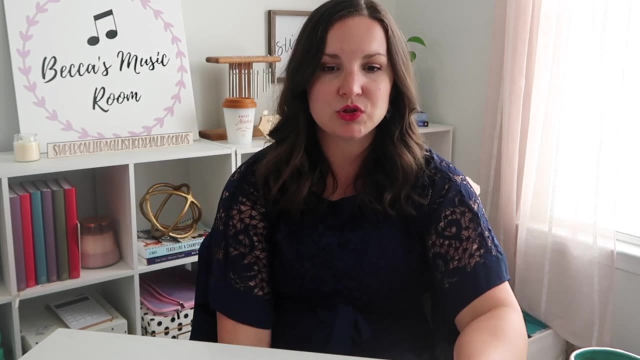 we get. some people do more rhythms, some people do less. it just kind of depends on how often you see your kids and all that stuff. please remember that all kids are different, all schools are different, so if you don't get through all of those rhythms like, it's okay, we didn't get through all. 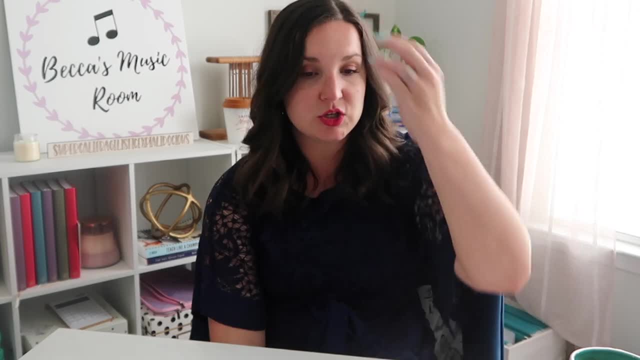 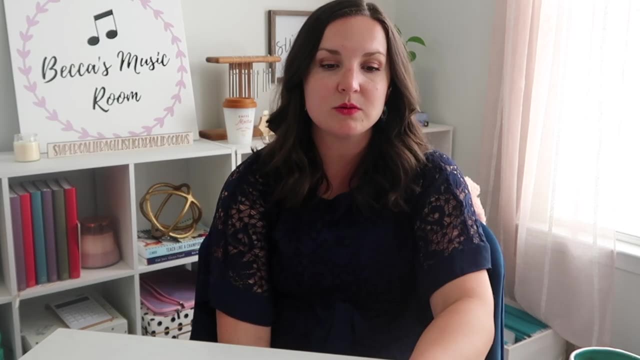 of those stuff, all that stuff at the beginning, and if i went to a new school, you know there's a lot of different rhythms and i'm not sure if the kids knew as much as i wanted them to do to know, or if they knew more than i want them to know, or any of that kind of stuff. 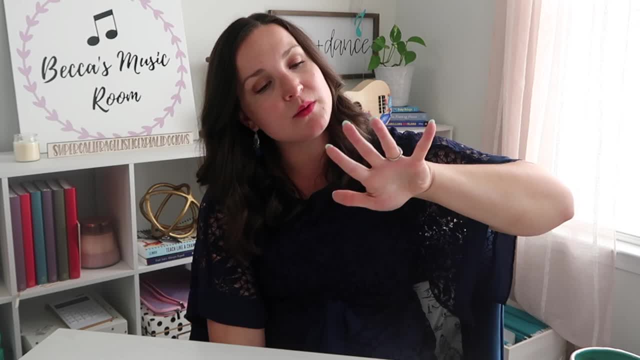 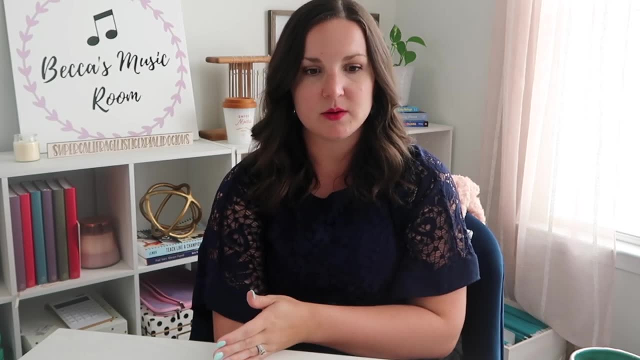 also remember that reading, identifying, writing, dictating and playing rhythms are all different things. so you want to make sure you hit all five of those concepts with each of the rhythms. so when you're doing half notes, you want to read half notes, identify half notes, write half notes. 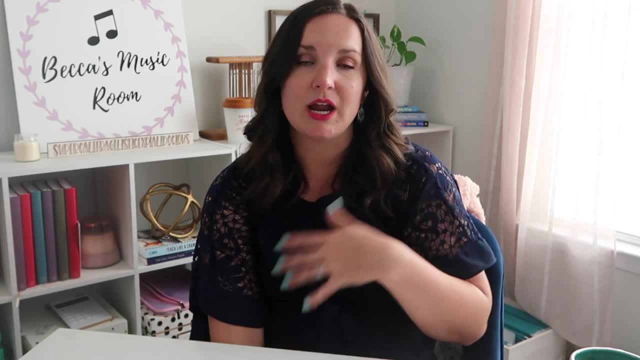 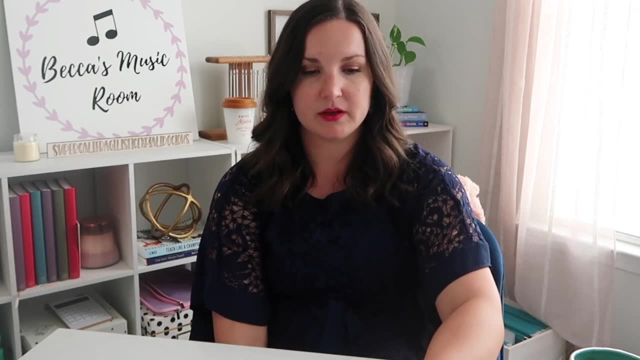 dictate half notes and you want to have them play half notes on your body, percussion or on actual instruments. these are all different skills to to make sure that they understand things fully. that's really going to help you. you really want to make sure that you get like all of that done.